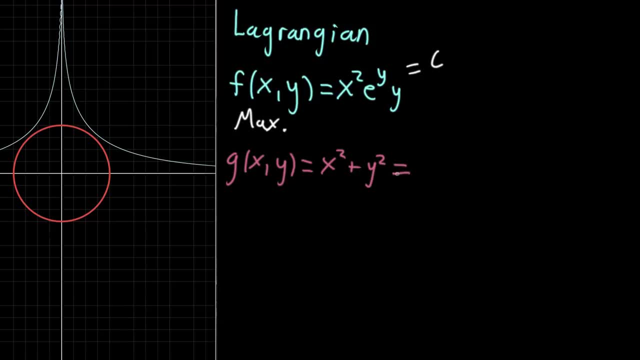 And we want to say that this has to equal some specific amount. In this case, I'm going to set it equal to 4.. So we say you can't look at any x, y to maximize this function. You are limited to the values of x and y that satisfy this property. 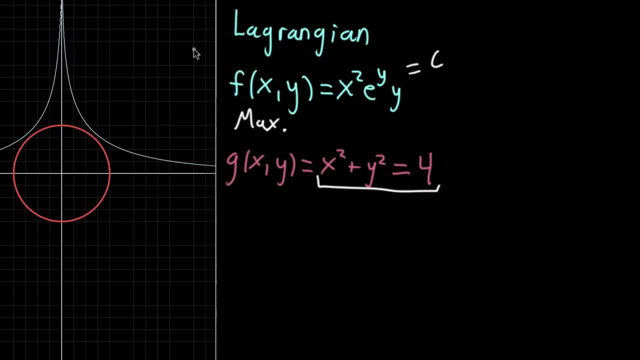 And I talked about this in the last couple videos and kind of the cool thing that we found was that you look through the various tables, different contour lines of f and the maximum will be achieved when that contour line is just perfectly parallel to this contour of g. 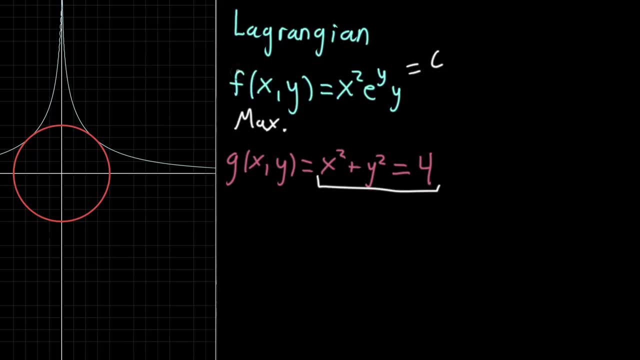 And you know, a pretty classic example for what these sorts of things could mean or how it's used in practice is if this was, say, a revenue function for some kind of company. You're kind of modeling your revenues based on different choices you could make running that company. 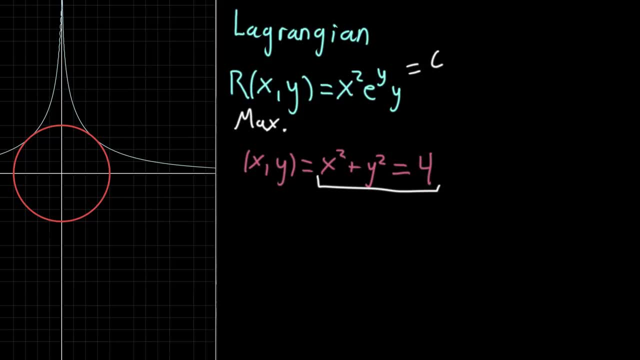 And the constraint that you'd have would be, let's say, a budget. So I'm just going to go ahead and write budget or b for budget here. So you're trying to maximize revenues and then you have some sort of dollar limit. 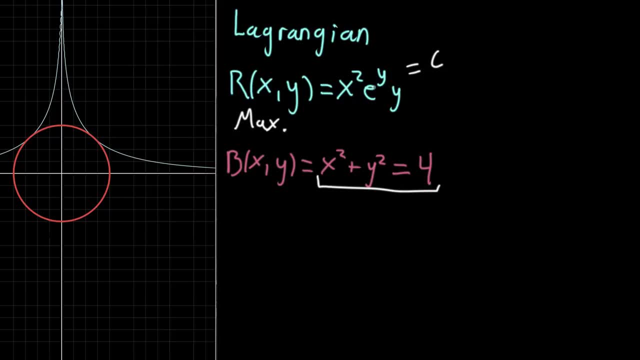 for what you're willing to spend, And these, of course, are just kind of made-up functions. You'd never have a budget that looks like a circle and this kind of random configuration for your revenue. But in principle, you know what I mean, right. 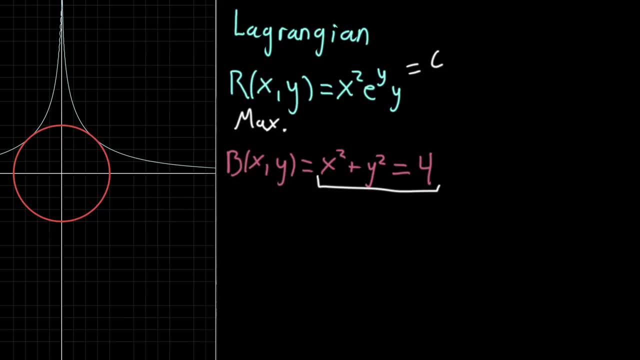 So the way that we took advantage of this tangency property- and I think this is pretty clever, let me just kind of redraw it over here- You're looking at the point where the two functions are just tangent to each other- is that the gradient vector for the thing we're maximizing? 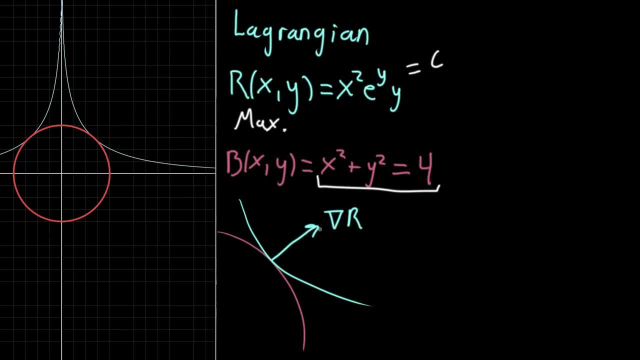 which in this case is r, is going to be parallel or proportional to the gradient vector of the constraint, which in this case is b. It's going to be proportional to the gradient of the constraint, And what this means is that if we were going to solve a set of equations, 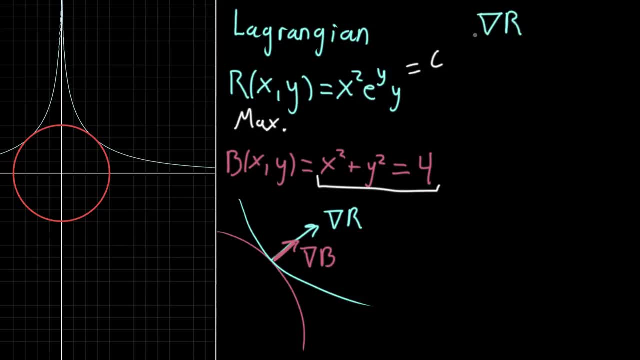 what you set up is you compute that gradient of r and it'll involve, you know, two different partial derivatives and you set it equal, not to the gradient of b, because it's not necessarily equal to the gradient of b, but it's proportional. 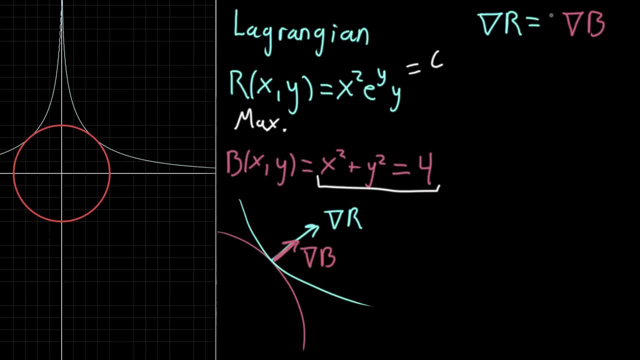 It's some kind of proportionality. constant lambda. Now let me, that's kind of a squirrely lambda Lambda. Yeah, that one doesn't look good either, does it? Why are lambdas so hard to draw? All right, that looks fine. 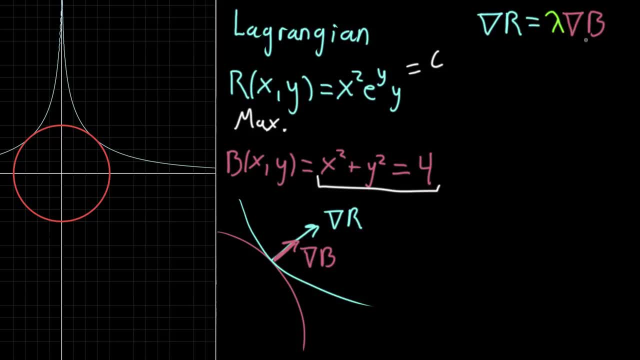 So the gradient of the revenue is proportional to the gradient of the budget, And we did a couple examples of solving this kind of thing. This gives you two separate equations from the two partial derivatives and then you use this right here, this budget constraint, as your third equation. 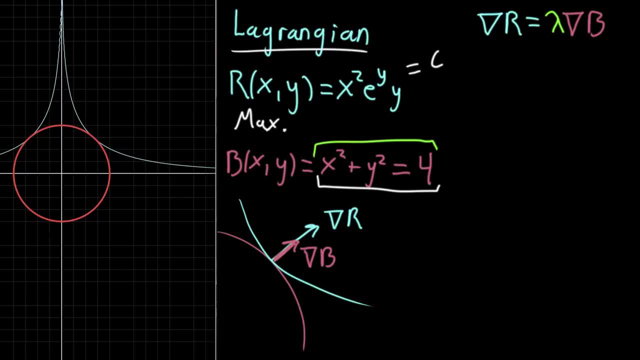 The Lagrangian, the point of this video. this Lagrangian function is basically just a way to package up this equation, along with this equation, into a single entity, So it's not really adding new information and if you're solving things by hand, 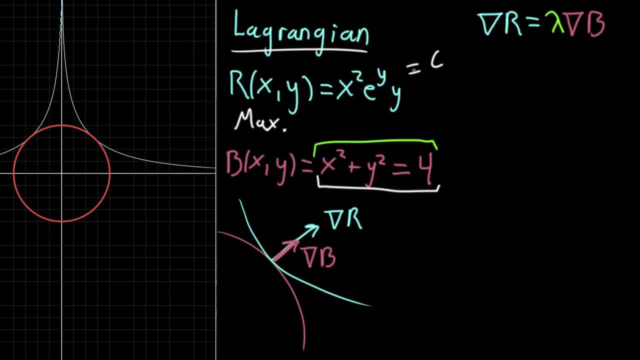 it doesn't really do anything for you. But what makes it nice is that it's something easier to hand a computer, and I'll show you what I mean. So I'm going to define the Lagrangian itself which we write with this kind of funky-looking script: L. 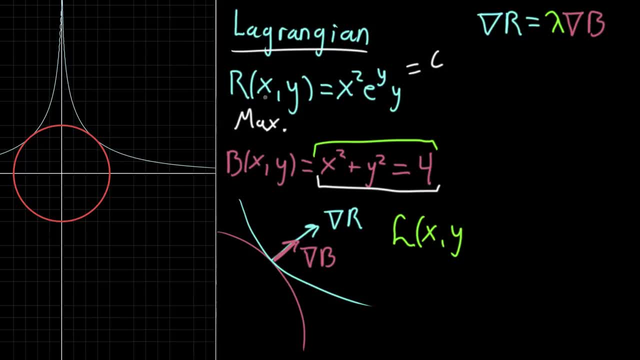 and it's a function with the same inputs that your revenue function or the thing that you're maximizing has, along with lambda, along with that Lagrange multiplier And the way that we define it, and I'm going to need some extra room. 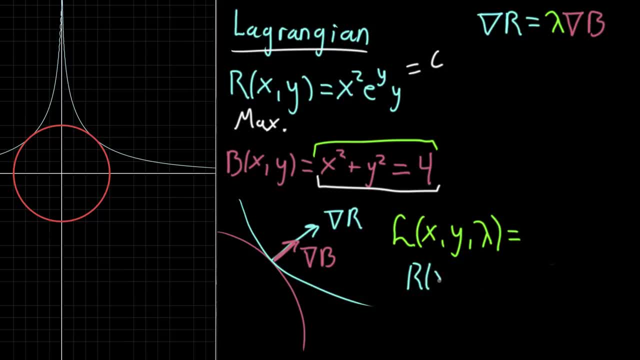 so I'm going to say it's equal to- and kind of define it down here- the revenue function or whatever it is that you're maximizing, the function that you're maximizing minus lambda, that Lagrange multiplier. so that's just another input to this new function. 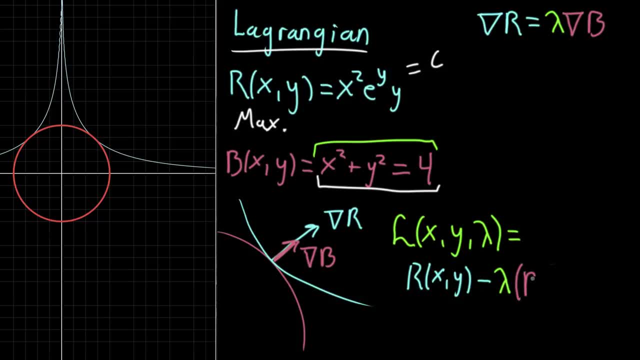 that we're defining, multiplied by the constraint function, in this case b, evaluated at x, y minus whatever that constraint value is. In this case, I put in four. so you'd write minus four If we wanted to be more general. 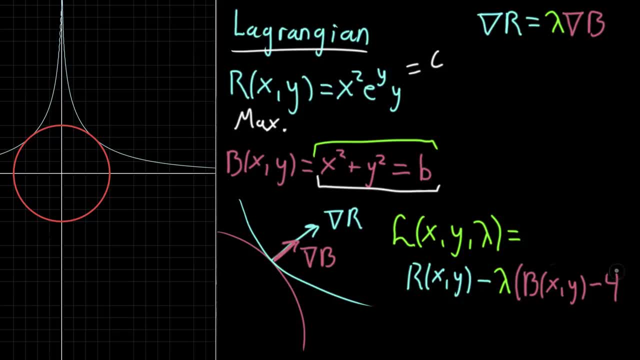 maybe we would write b for whatever your budget is. so over here you're subtracting off little b. So this here is a new multivariable function. right, It's something where you could input x, y and lambda and just kind of plug it all in. 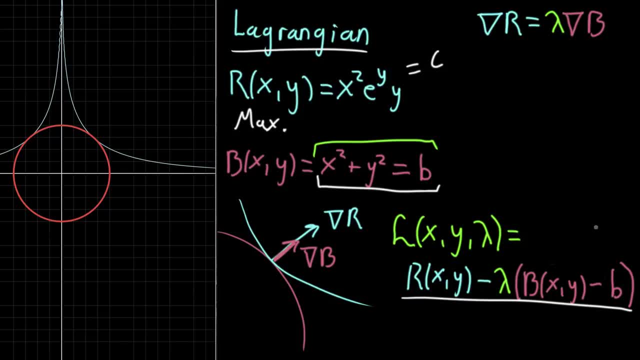 and you'd get some kind of value. And remember, b in this case, is a constant, so I'll go ahead and write that, that this right here is not considered a variable. this is just some constant. Your variables are x, y and lambda. 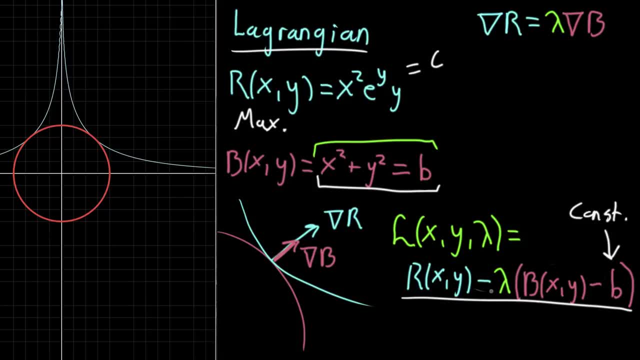 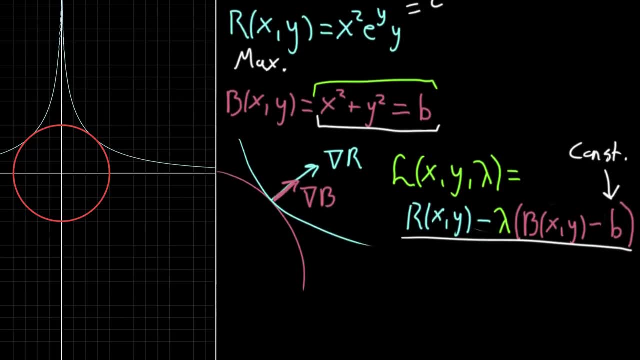 And this would seem like a totally weird and random thing to do if you just saw it out of context or if it was unmotivated. but what's kind of neat- and we'll go ahead and work through this right now- is that when you take this: 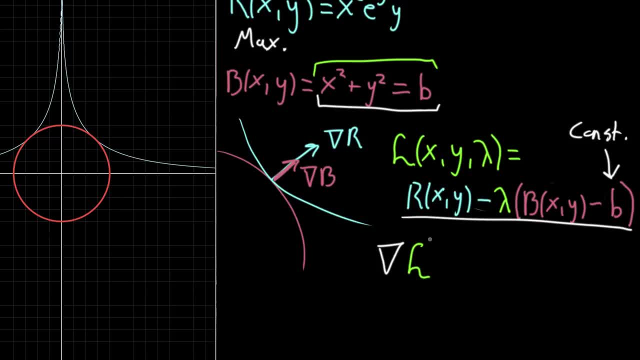 is that when you take the gradient of this function called the Lagrangian and you set it equal to zero, that's going to encapsulate all three equations that you need, And I'll show you what I mean by that. So let's just remember the gradient of L. 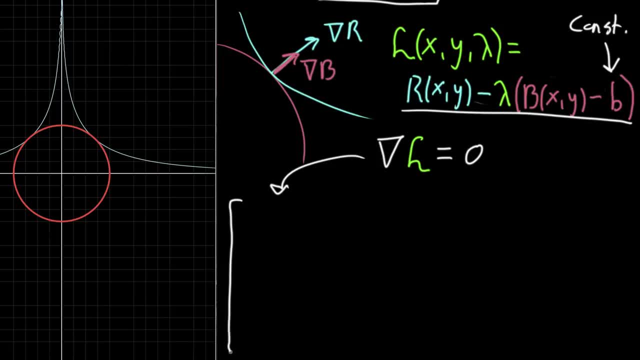 that's a vector. It's got three different components, since L has three different inputs. You're going to have the partial derivative of L with respect to x, You're going to have the partial derivative of L with respect to y And then, finally, the partial derivative of L. 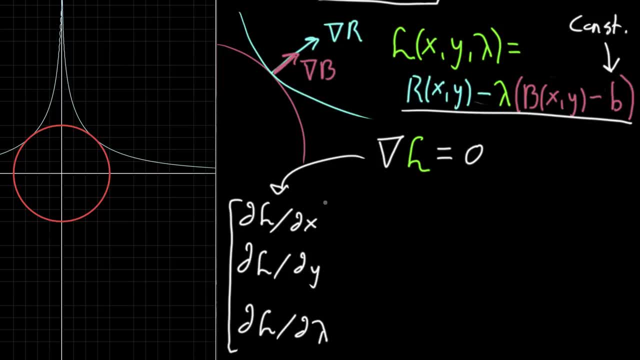 with respect to lambda, which is the Lagrange multiplier which we're considering an input to this function, And remember, whenever we write that a vector equals zero, really we mean the zero vector. Often you'll see it in bold if it's in a textbook. 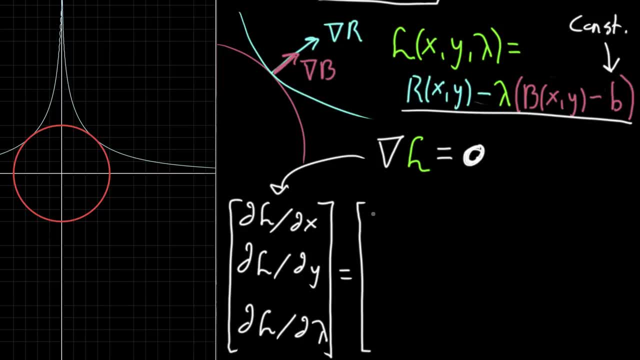 but what we're really saying is we set those three different functions, the three different partial derivatives all equal to zero. So this is just a nice closed form, compact way of saying: set all of its partial derivatives equal to zero And let's go ahead and think about: 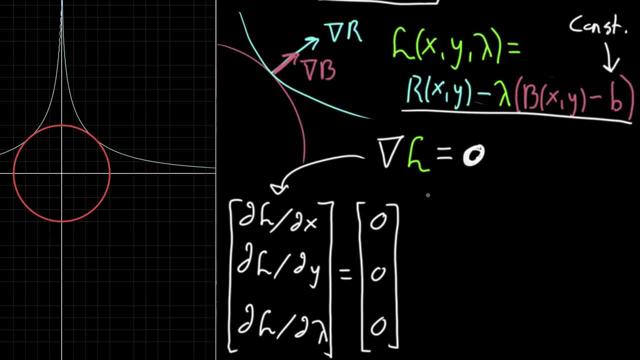 what those partial derivatives actually are. So this first one, the partial with respect to x, partial derivative of the Lagrangian with respect to x. It's kind of fun, you know. you have all these curly symbols, the curly d, the curly l. 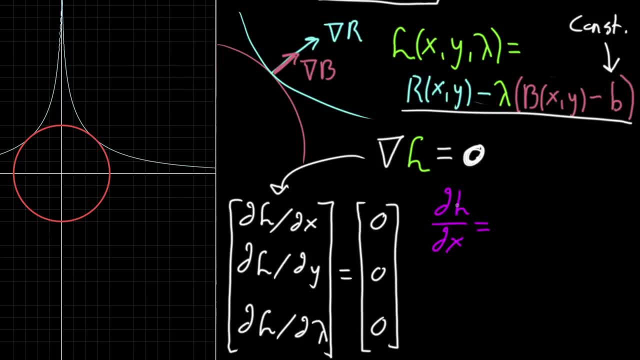 it makes it look like you're doing some truly advanced math, But really it's just kind of artificial fanciness, right? But anyway. so we take the partial derivative with respect to x, and what that equals is- well, it's whatever. the partial derivative of r. 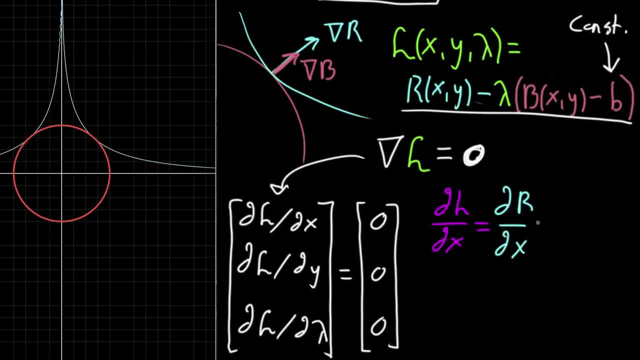 with respect to x is minus, and then lambda. from x's perspective, lambda just looks like a constant. So it's going to be lambda. And then this, inside the parentheses, the partial derivative of that with respect to x. well, it's going to be whatever. 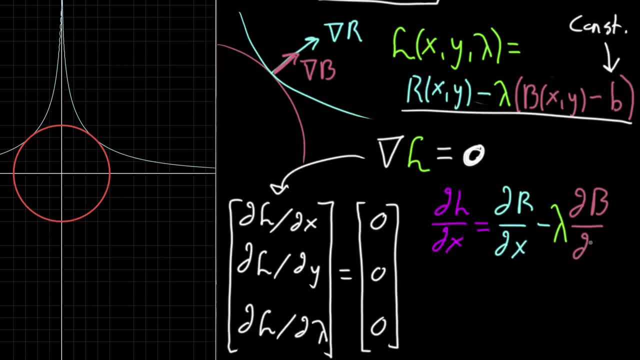 the partial derivative of b is with respect to x. But subtracting off that constant that doesn't change the derivative. So this right here is the partial derivative of lambda with respect to x. Now, if you set that equal to zero- and I know I've kind of run out of room on the right here- 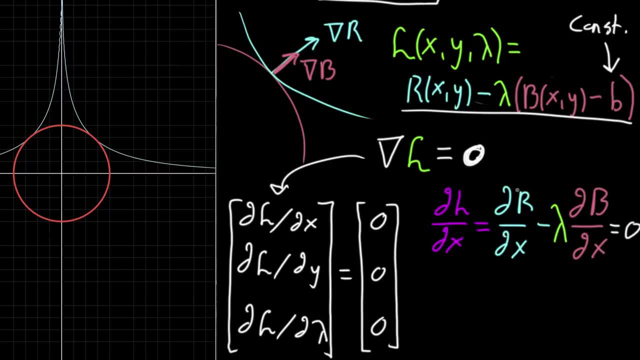 but if you set that equal to zero, that's the same as just saying that the partial derivative of r with respect to x equals lambda times the partial derivative of b with respect to x. And if you think about what's going to happen when you unfold this property, 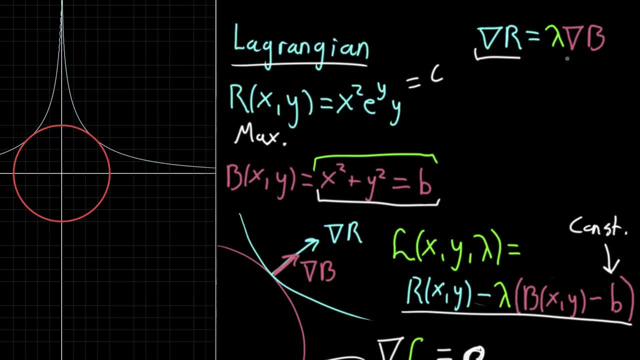 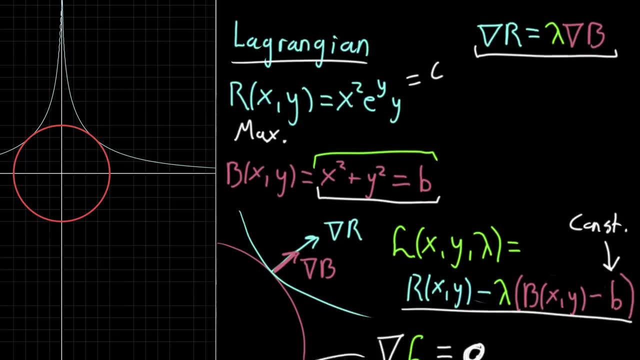 that the gradient of r is proportional to the gradient of b, written up here. that's just the first portion of this right. If we're setting the gradients equal, then the first component of that is to say that the partial derivative of r with respect to x. 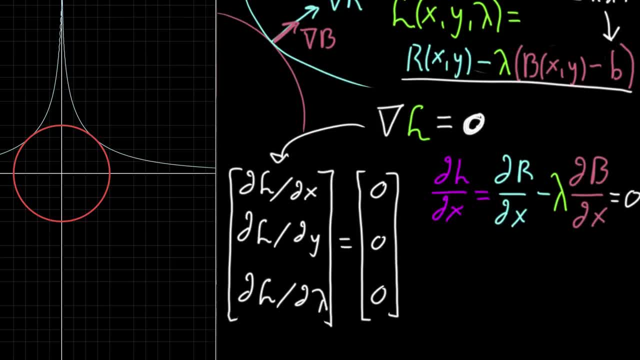 is equal to lambda times the partial derivative of b with respect to x. And then, if you do this for y, if we take the partial derivative of this Lagrangian function with respect to y, it's very similar. right, It's going to be well, you just take. 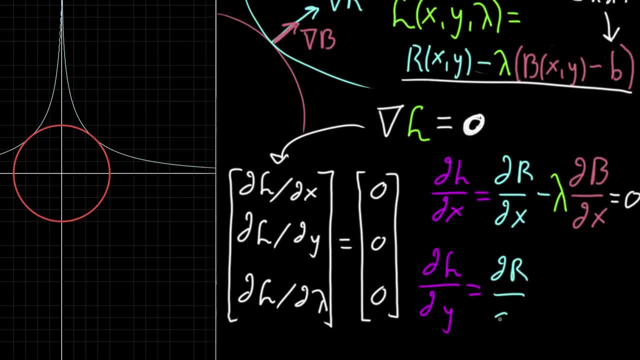 the partial derivative of r with respect to y. In fact, it all looks just identical. Whatever r is, you take as partial derivative with respect to y, and then we subtract off. lambda looks like a constant as far as y is concerned. 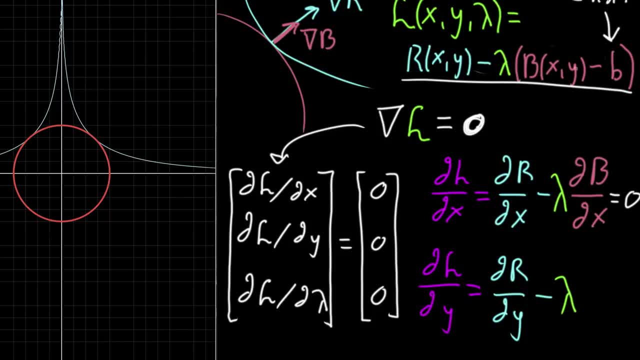 and then that's multiplied by well, what's the partial derivative of this term, inside the parentheses, with respect to y? Well, it's the partial of b with respect to y, And again, again, if you imagine setting that equal to zero. 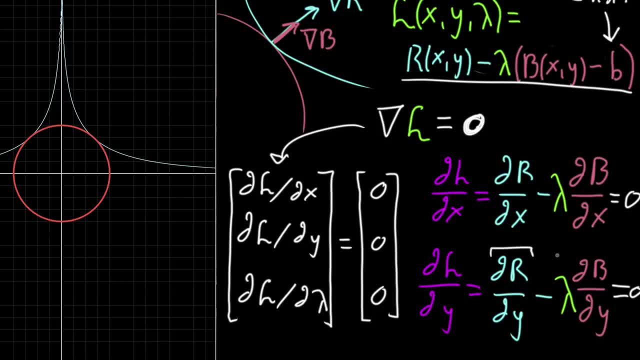 that's going to be the same as setting this partial derivative term equal to lambda times this partial derivative term right, You kind of just bring one to the other side. So this second component of our Lagrangian equals zero equation is just the second function. 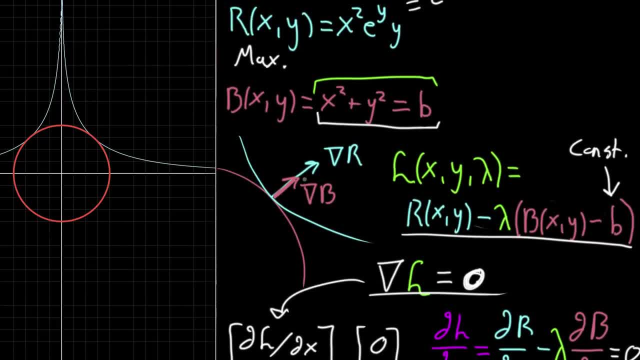 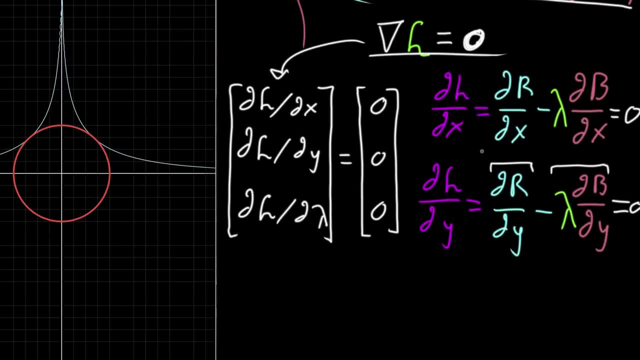 that we've seen in a lot of these examples that we've been doing, where you set one of the gradient vectors proportional to the other one, And the only real difference here from stuff that we've seen already- and even then it's not that different. 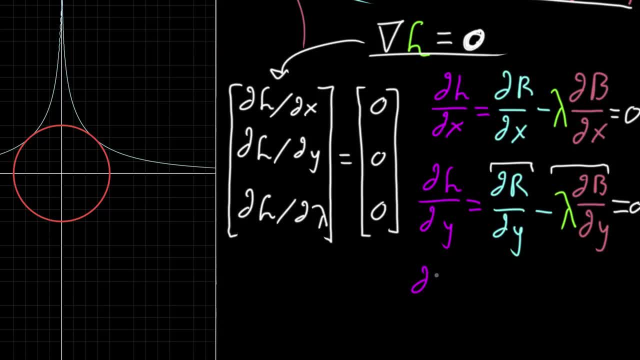 is that what happens when we take the partial derivative of this Lagrangian with respect to lambda? with respect now I'll go ahead and give it that kind of green lambda color here. Well, when we take that partial derivative, if we kind of look up at the definition of the function, 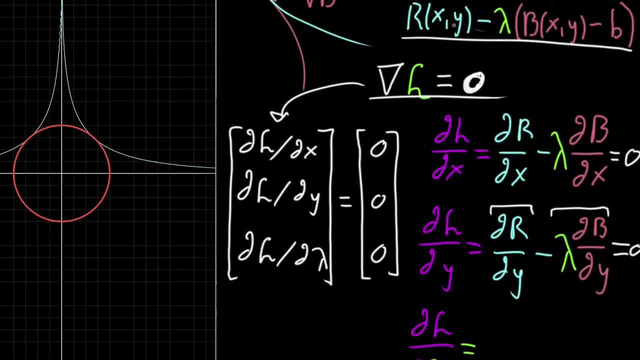 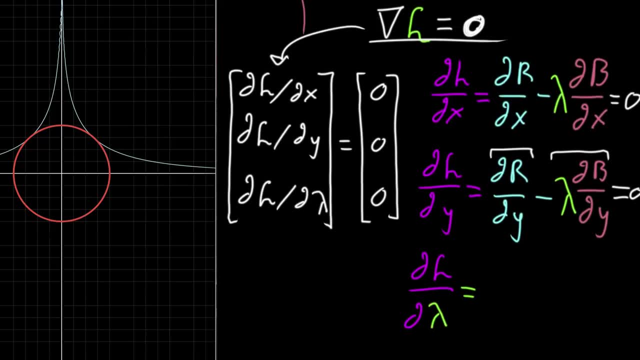 r, r never has a lambda in it right? It's purely a function of x and y, So that looks just like a constant when we're differentiating with respect to lambda. So that's just going to be zero when we take its partial derivative. 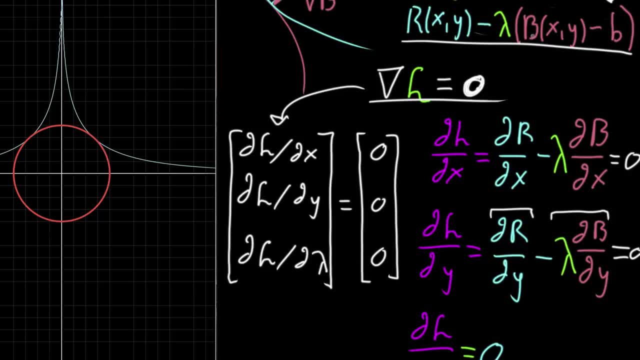 And then this next component b of xy minus b. all of that just looks like a constant as far as lambda is concerned. right, There's x's, there's y, there's this constant b, but none of these things have lambdas in them. 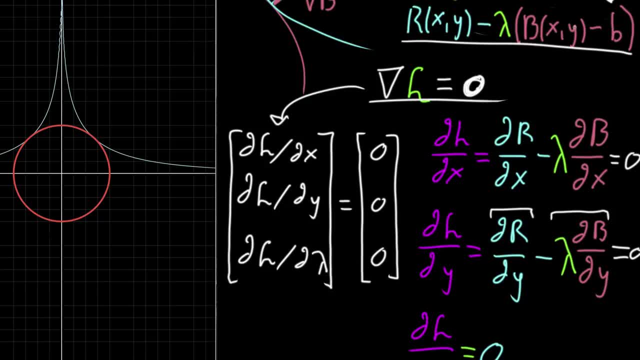 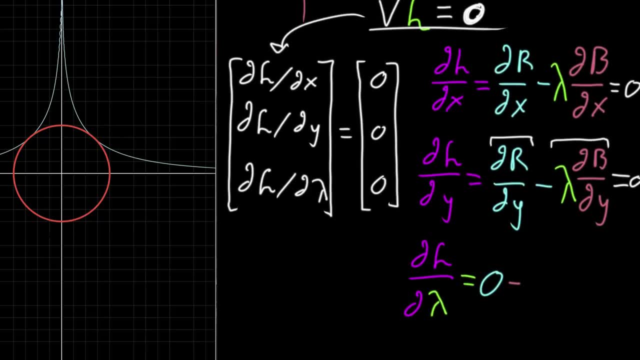 So when we take the partial derivative with respect to lambda, this looks like some big constant times lambda itself. So what we're going to get is: I guess we're subtracting off right. It's up here kind of writing, a minus sign. 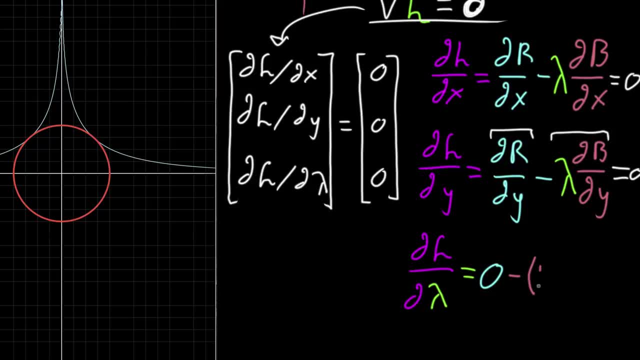 We're subtracting off all the stuff that was in those parentheses: b of xy minus b, that constant And this whole thing. if we set that whole thing equal to zero, well that's pretty much the same as setting b of xy minus b equal to zero. 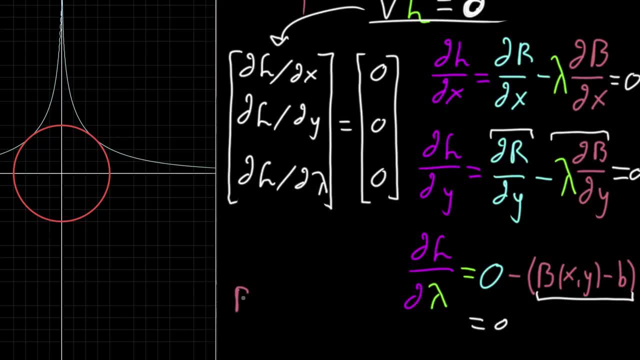 And that's really just the same as saying: hey, we're setting b of xy equal to that little b right. Setting this partial derivative of the Lagrangian with respect to the Lagrange multiplier equal to zero boils down to the constraint right. 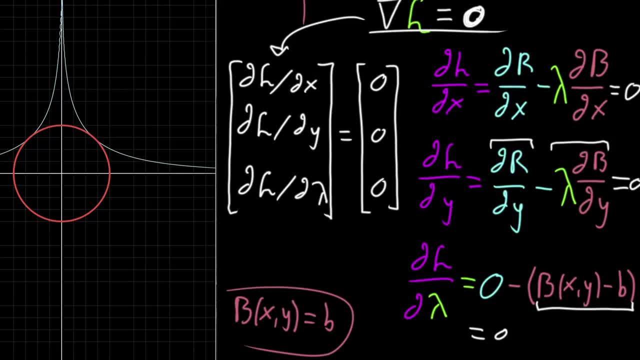 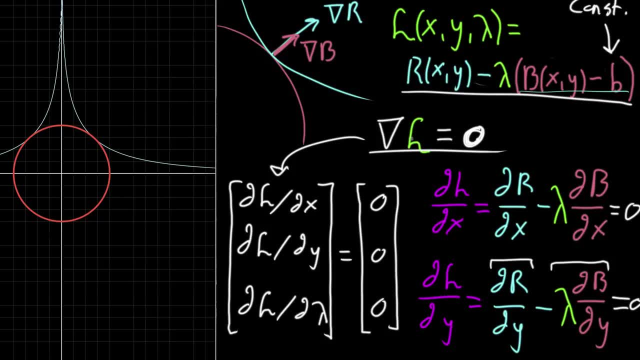 The third equation that we need to solve. So in that way, setting the gradient of this Lagrangian function equal to zero is just a very compact way of packaging three separate equations that we need to solve- the constraint optimization problem, And I'll emphasize that in practice, 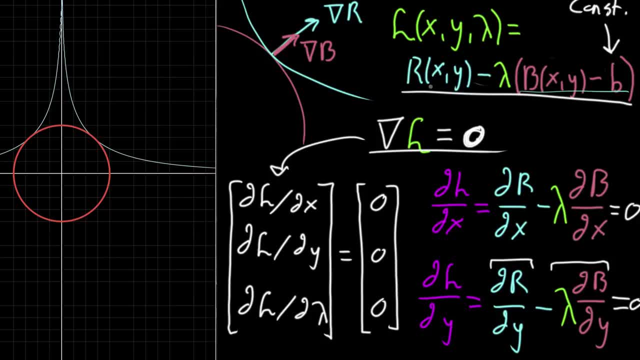 if you actually see a function for r, for the thing that you're maximizing, and a function for the budget, it's much better, I think, to just directly think about these parallel gradients and kind of solve it from there. Because if you construct the Lagrangian, 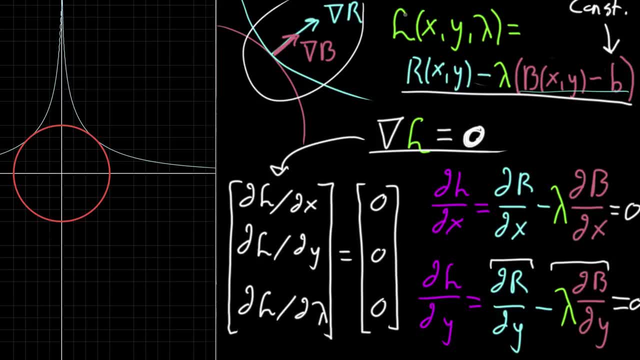 and then compute its gradient. all you're really doing is repackaging it up, only to unpackage it again. But the point of this kind of the reason that this is a very useful construct is that computers often have really fast ways of solving things like this. 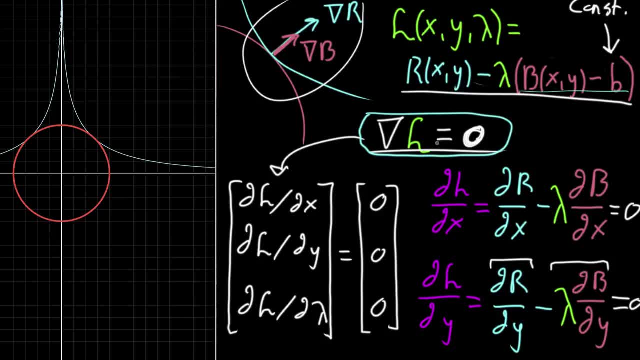 things like the gradient of some function equals zero, And the reason is because that's how you solve unconstrained maximization problems, right? This is very similar to as if we just looked at this function l out of context and were asked: hey, what is its maximum value?